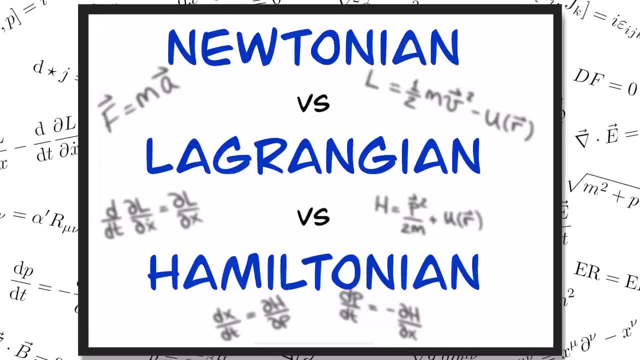 physics class when they learn to apply F equals ma to simple systems. But there are two other formulations of mechanics that are actually more widely used by modern physicists, and they're essential for understanding quantum mechanics, meaning the physics of very small objects like elementary particles. These are the Lagrangian and Hamiltonian formalisms of mechanics. 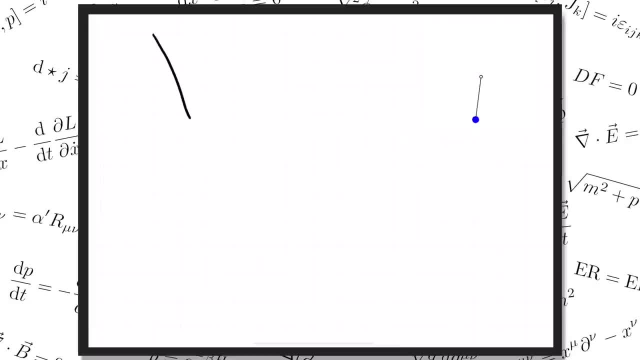 and in this video I'm going to teach you the basics of both. I'm going to illustrate each approach using the simple pendulum as an example. So we've got a particle of mass m hanging from a lightweight rod of length l which is attached to a pivot at its other end. Now I'll assume that 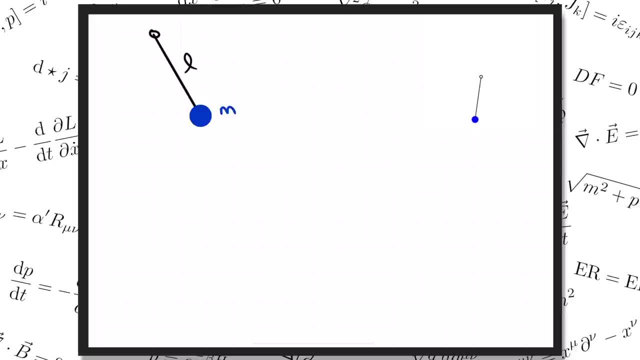 you've already learned how to analyze a pendulum using. F equals ma, so I'm only going to review that briefly right now. but if you're interested in learning more about quantum mechanics, you can click the link in the description below. But I've posted a whole other video. 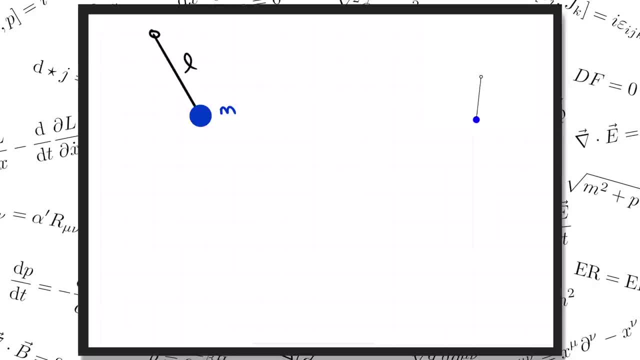 just reviewing the basics of pendulums that I'll link below so you can check that out if you want to see more of the details, And I'll also paste a link to some notes that I wrote about these topics which you might also want to check out after you've watched this video. 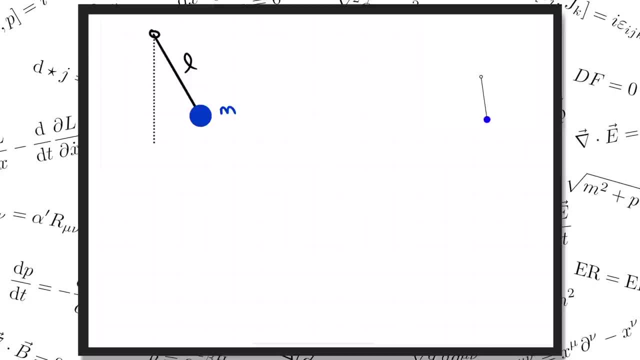 First of all, we need to set up some coordinates to describe the position of the pendulum. We can use whatever coordinates we want, but it's simplest to use either the arc length coordinate s that runs along the circumference of the circle traced out by the particle. 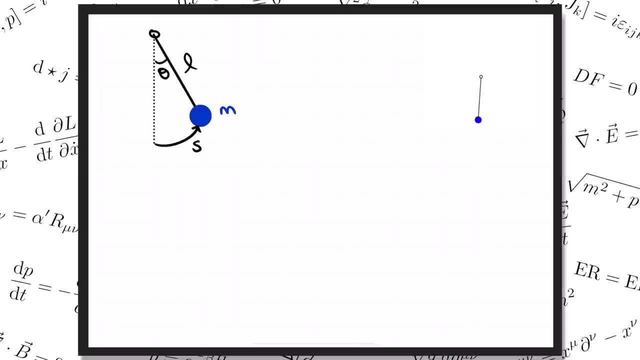 or we can use the angle that the rod makes with the vertical theta. They're totally equivalent and either one will do the job for specifying the position of the mass. The relation between them is just the definition of the angle theta. in radians It's the arc length s divided by the 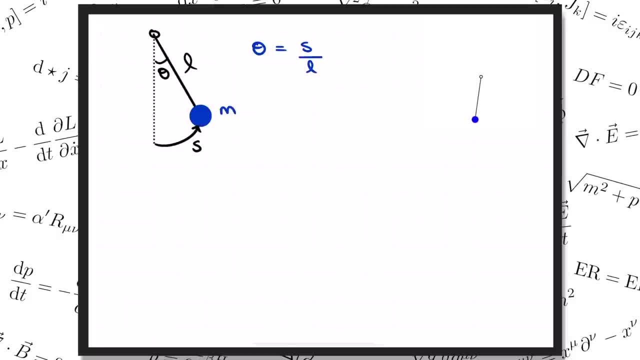 radius l. We want to predict how the pendulum is going to move when you pull it up to some initial angle and let it go, or if you were to give it a little kick. According to Newton, we should start by writing down all the forces that are acting on the particle. There's only two. 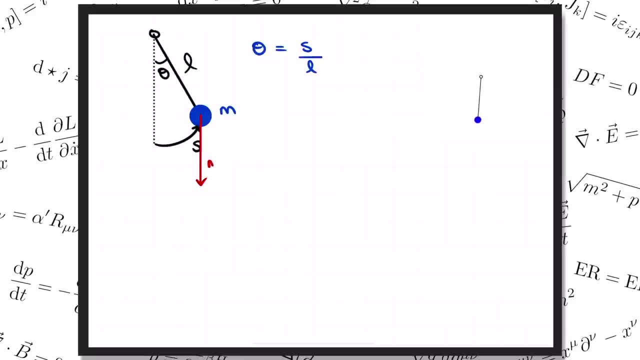 of these Gravitational angle, angle theta and angle theta, We can use the angle that the rod is pointing at and the gravity mg pointing straight down and the tension t in the rod pulling radially back toward the center of the circle. Then Newton tells us to add up all the 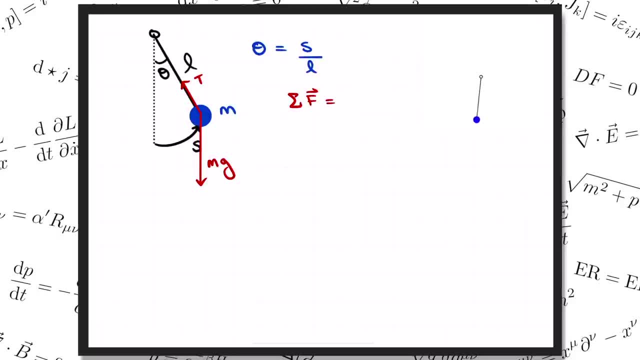 forces and write: F equals ma, The total force equals the mass times, the acceleration, F equals ma is a vector equation. but what we're really interested in here is the tangential component, meaning the component of the force and the acceleration that point along the circle where 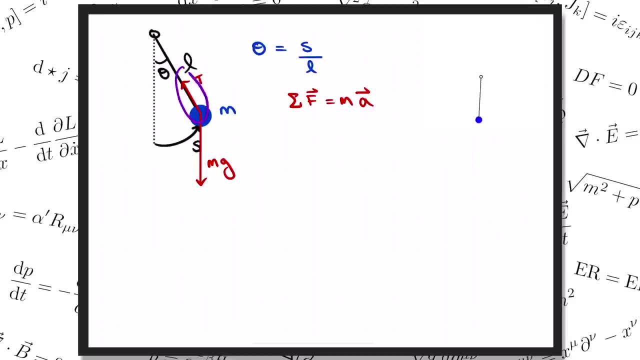 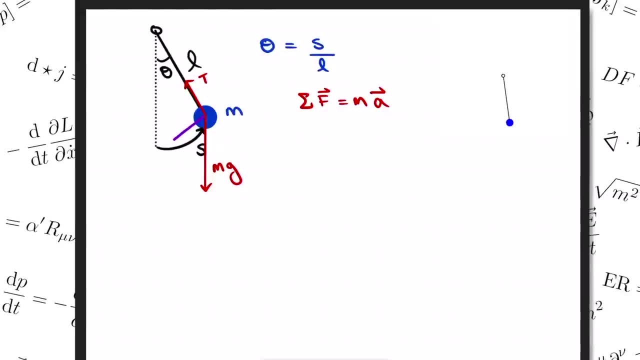 the particle is constrained to move. The tension isn't contributing anything here. That's pointing straight toward the center of the circle, which is perpendicular to the tangent direction. So the only relevant force is actually the tangential component of gravity. With a little geometry work. 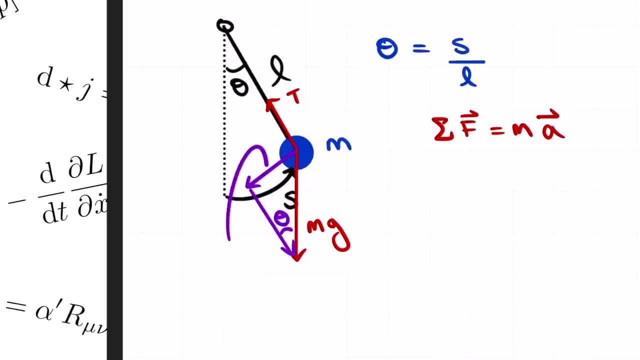 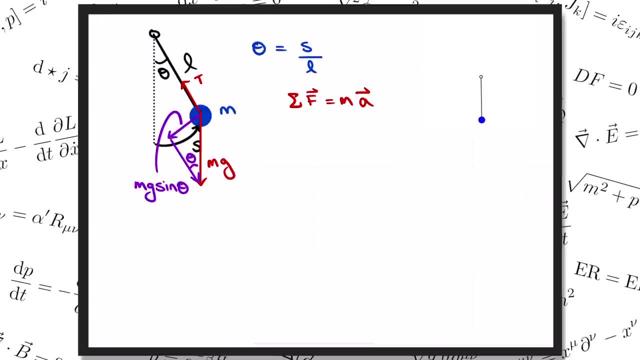 you can see, this is mg sine theta, pointing back toward the pendulum's equilibrium position. So F equals ma. for the arc length coordinate, s simply reads: m. s double dot equals minus mg sine theta. I'm using dots here to denote rates of change with respect to time. So if s of t is the 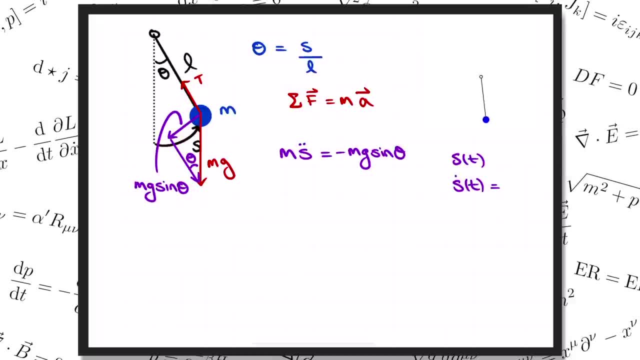 position as a function of time, then s dot equals d s by d. t is the velocity and s double dot is the acceleration, the second derivative of s with respect to time. I want to write everything in terms of theta, though, so I'm going to use the fact that s double dot is equal to L times theta. 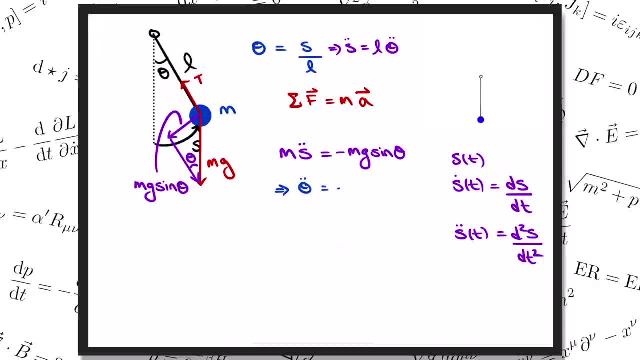 double dot. in order to rewrite the F equals ma equation, I'm going to use the fact that s double dot equals ma equation as theta double dot equals minus g over L sine theta. This is called the equation of motion for theta, It's the differential equation that governs the motion of the pendulum. 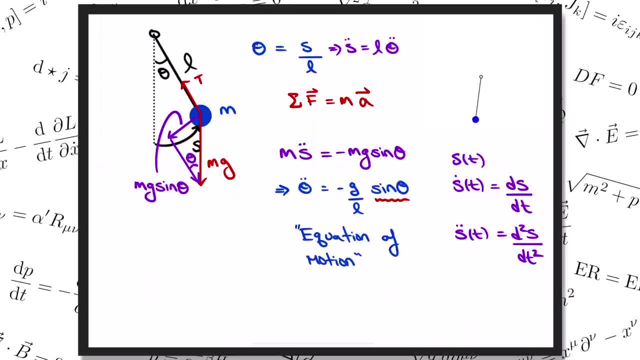 And it's actually pretty complicated in this case because of this factor of sine theta on the right hand side. Too complicated, in fact, for us to be able to write down a simple solution in general. There is one special case when we can, though, and that's when theta is small. 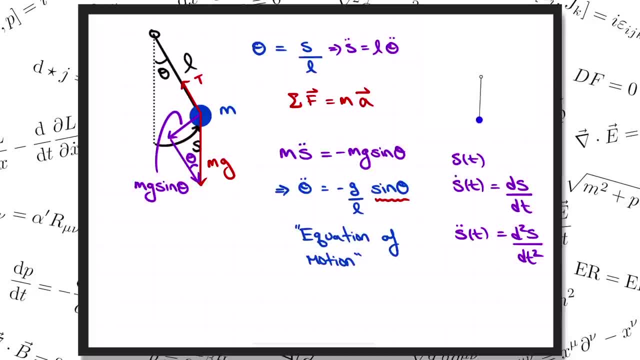 meaning that the pendulum never gets very far away from its equilibrium position. In that case, the solution is just a sine or cosine. If you want to know how that works, check out the other video that I posted, all about pendulums, that I've linked down below. 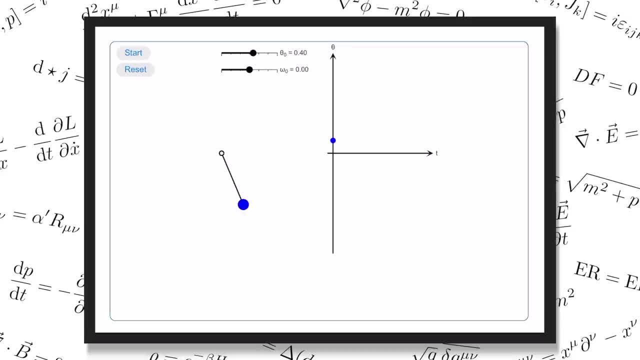 Here's a little animation that I made to show you what this looks like. I'll paste a link below so you can go play with it too. You drag these little sliders here to set the initial angle and initial angular speed of the pendulum and then press start to let it go and see the resulting motion. 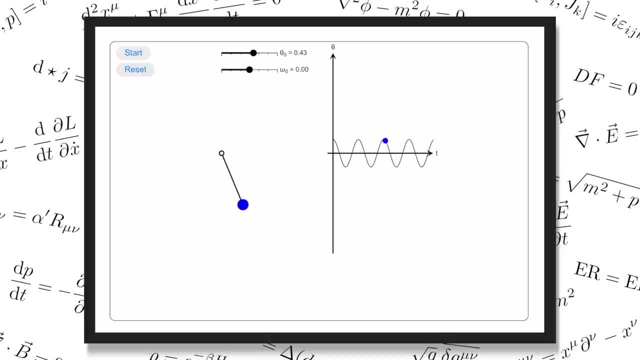 When I release it from a small angle like this, you can see that theta versus t indeed looks like a cosine function. So I hope you'll go play with this. Try choosing different values for the initial conditions by dragging those sliders. Draw for yourself what you think. the graph of theta versus 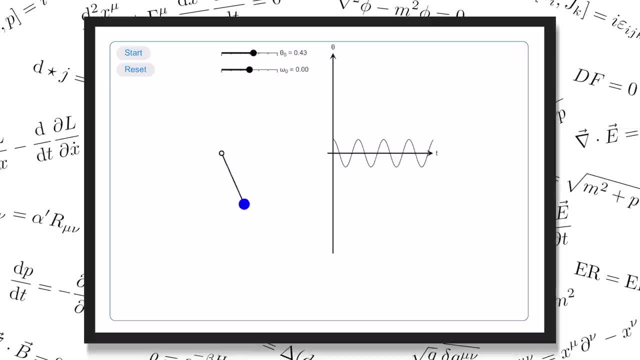 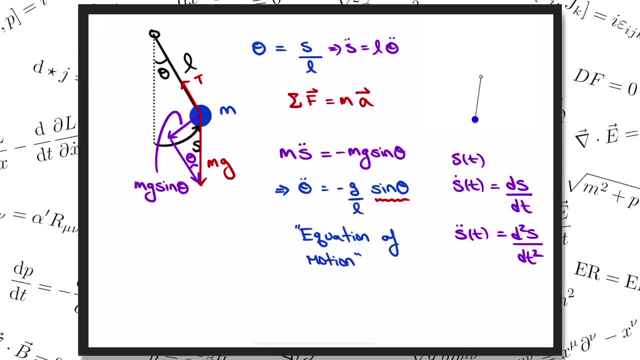 t should look like with those initial conditions and then press start to see if you got it right. All right, so that's a quick review of how we understand the motion of the pendulum using Newtonian mechanics and F equals ma, But there's a lot more to mechanics than F equals ma. 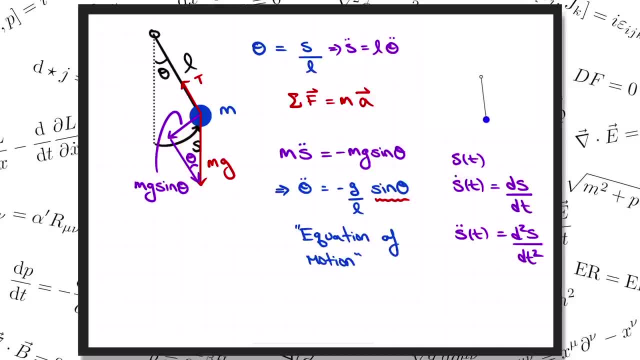 and in the years after Newton's work. in the late 1600s, new approaches to mechanics were developed by Joseph-Louis Lagrange. in the late 1700s, In the late 1800s, Newton's work was developed by Joseph-Louis. Lagrange in the late 1700s, In the late 1900s. Newton's work was developed by Joseph-Louis Lagrange in the late 1700s, In the late 1900s. Newton's work was developed by Joseph-Louis Lagrange in the late 700s. 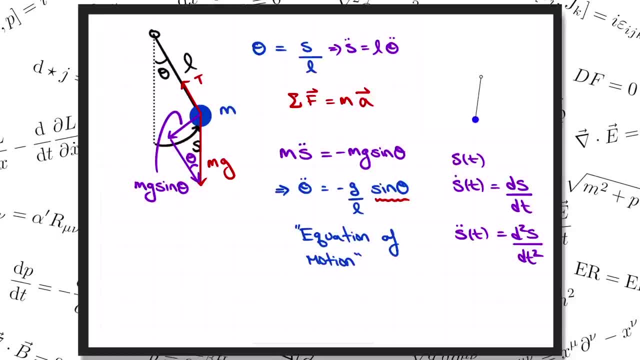 In the late 1700s. Newton's work was developed by Joseph-Louis Lagrange in the late 700s And by William Rowan Hamilton in the 1800s. Lagrange and Hamilton's approaches offer new practical and theoretical insights into the structure of mechanics, And they're especially 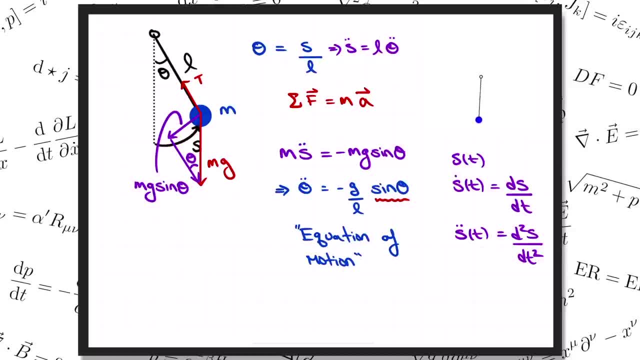 relevant in the study of quantum mechanics, meaning the physics of very small objects like atoms and elementary particles, as opposed to the classical mechanics that Newton, Lagrange and Hamilton originally studied. Now, I should say that the Lagrangian and Hamiltonian 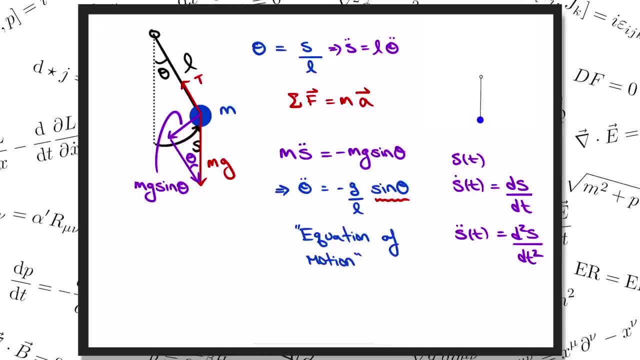 approaches to mechanics are a little bit more mathematically sophisticated than Newton's approach, So depending on how much math you've already learned, they might seem like they're a little bit more challenging. But they're both really fascinating and they provide new insights and 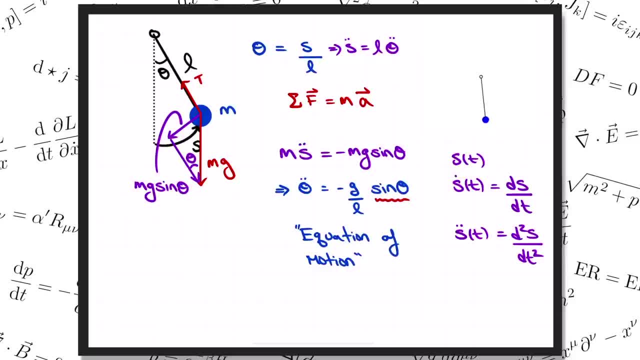 strategies for solving problems. Remember that it's also totally fine if you don't follow every single detail that I present here. What I'm really hoping is that you'll be inspired to go off and keep learning more on your own. Alright, let's look at the Lagrangian formalism next. Whereas 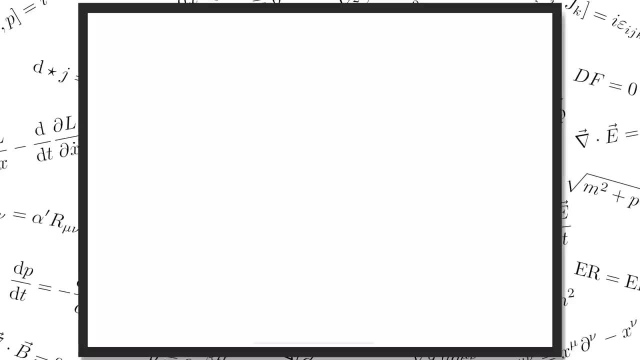 Newton told us to start by writing down the total force. Lagrange tells us to start by writing down the potential energy and then taking their difference. This defines a function called the Lagrangian L. Let's see what the Lagrangian is for our pendulum example: The kinetic energy k. 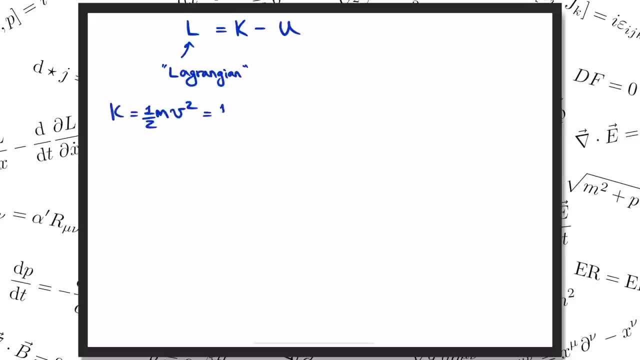 is, of course, just one half mv squared. where v equals s, dot is the speed of the particle. Actually, I'd like to write everything in terms of theta, so I'm going to replace s dot with L times theta dot. Then the kinetic energy is one half m L squared theta. 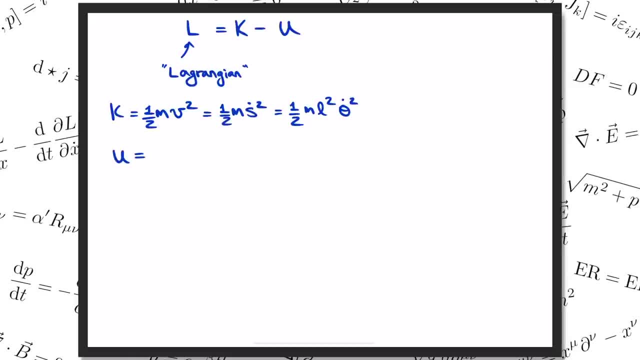 The potential energy u, meanwhile, is just mg times y the height of the particle above some chosen ground level. I'm going to put ground level at the height of the pivot. Then the y-coordinate of the particle is minus L cosine theta and the potential energy is minus mg L cosine theta. 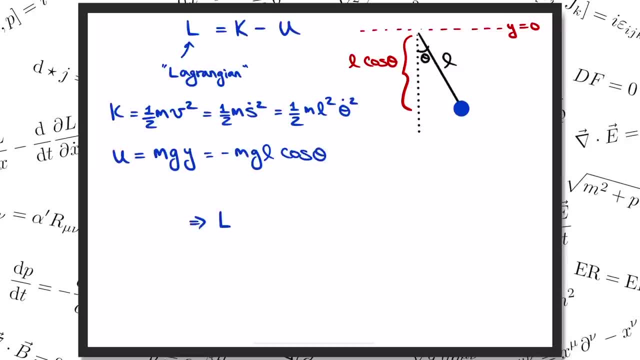 So the Lagrangian for our pendulum is the difference between the kinetic energy and potential energy. That's one half m L squared theta dot. So Newton told us to start by writing the total force and setting it equal to ma. Lagrange instead tells us to start by writing the Lagrangian, like we have here. 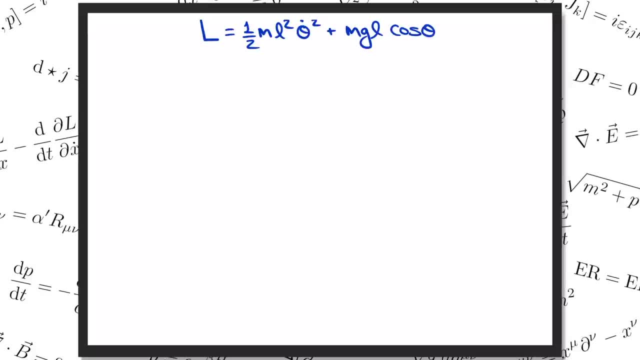 and then using it to write what's called the Euler-Lagrange equation, That's d by dt of dL by d theta. dot equals dL by d theta. The Euler-Lagrange equation can be written like this. By the way, the curly d's here stand for partial derivatives. 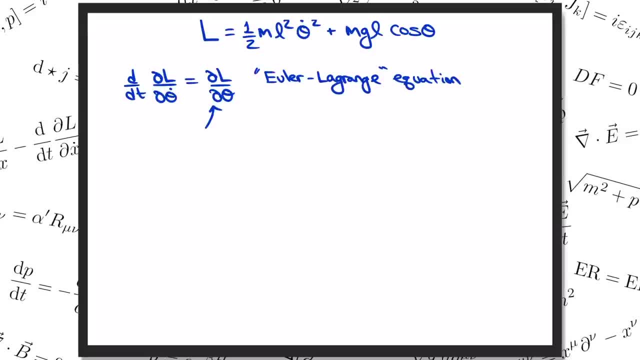 If you've never seen those before, don't worry about it. For practical purposes they behave just like ordinary derivatives. Now I'm not going to get into too much motivation as to where this Euler-Lagrange equation comes from in this video. What I just want to do for 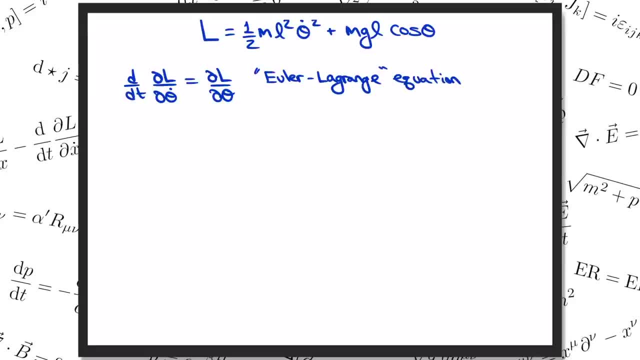 now is write it down and investigate the consequences. But the short answer is that the Euler-Lagrange equation is the condition for the action s to be minimized. where the action is defined as the integral of the Lagrangian, The claim is that, of all the possible paths that a particle could follow, 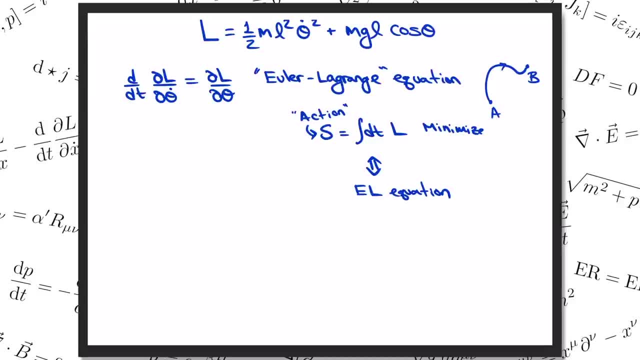 the one it actually chooses is the path that minimizes, or, more precisely, extremizes the action. This is known as the principle of least action, and the implication is that the trajectory satisfies the Euler-Lagrange equation. But unpacking all of those details would really require its own dedicated video. 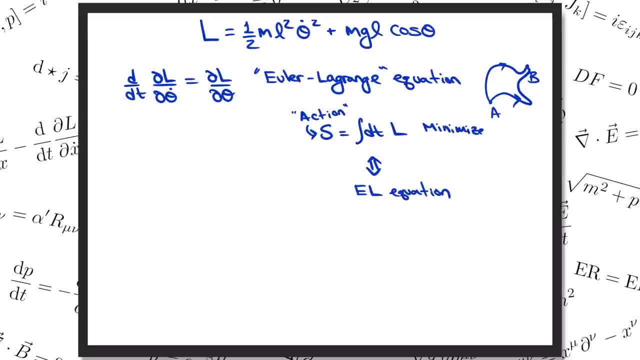 Right now. I just want to see what happens when we plug the pendulum Lagrangian into this Euler-Lagrange equation. The right hand side of the Euler-Lagrange equation is the derivative of L with respect to theta, And we're going to treat theta and theta dot as independent variables when we take these. 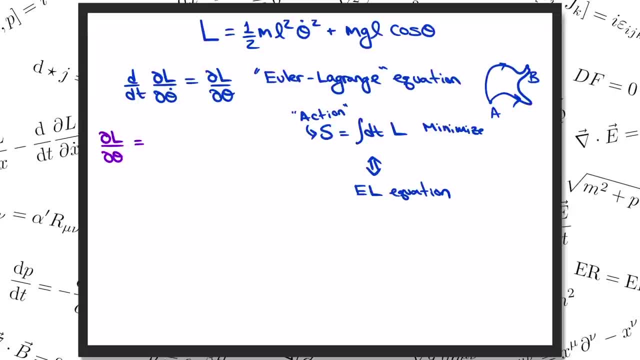 derivatives. That means that the only contribution to dl by d theta comes from the cosine theta term in the Lagrangian And we get dl by d theta equals minus mgl sine of theta. For the left hand side we need to know what dl by d theta dot is and from the kinetic energy term we get ml squared theta dot. 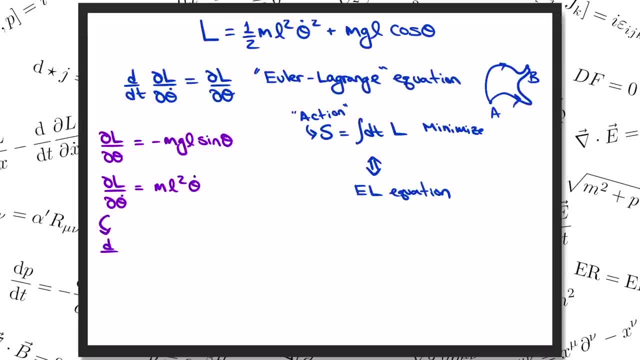 Then taking d by dt of that just turns theta dot into theta double dot. By the way, dl by d theta dot here is called the momentum p corresponding to the coordinate theta. dl by d theta is called the generalized force, The reason for the terminology. 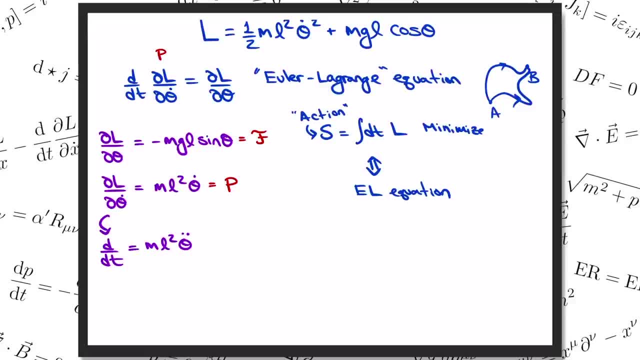 is that the Euler-Lagrange equation is then reminiscent of Newton's. second law Force is the rate of change of momentum. So the result of plugging in our pendulum, Lagrangian into the Euler-Lagrange equation says that ml squared theta double dot equals minus mgl sine. 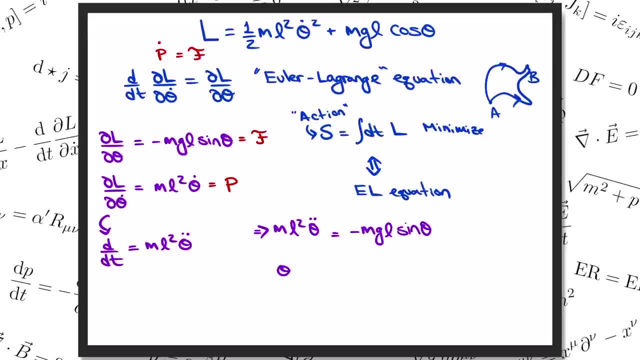 theta. Canceling out the common factors, we once again obtain theta. double dot equals minus g over l sine theta. The same equation of motion we obtained earlier using f equals ma, but this time we got it using a very different strategy, based on the Lagrangian and the Euler-Lagrange. 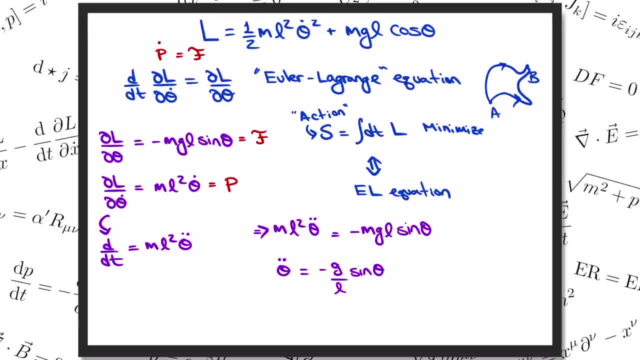 equation. All that might seem a little bit abstract if you've never encountered a Lagrangian before. It's a very useful way of quickly getting at the equations of motion for a system, often times easier than using f equals ma If I'm faced with most any mechanics problem, 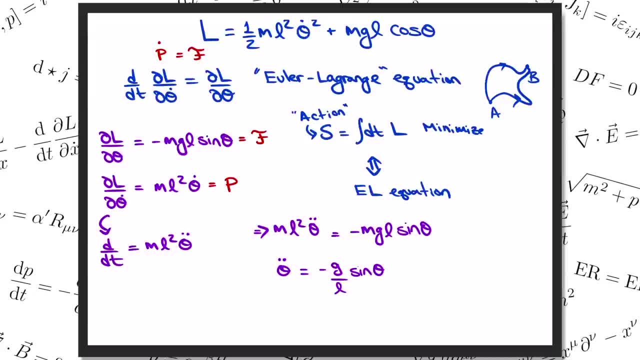 I'll usually start by writing down the Lagrangian. For one thing, we don't have to deal with any of the annoying vectors that show up in f equals ma. We can just choose whatever coordinates we like to describe our system, including potentially non-inertial coordinates. 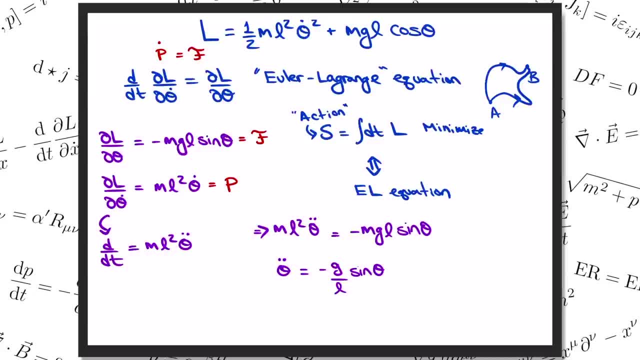 write down the Lagrangian and then write the Euler-Lagrange equation for each of the coordinates. The Lagrangian formalism also makes it much easier to deal with constraints and to understand symmetries, But those topics will have to wait for another day. 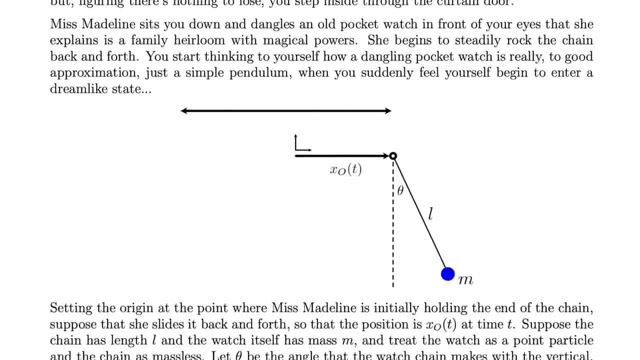 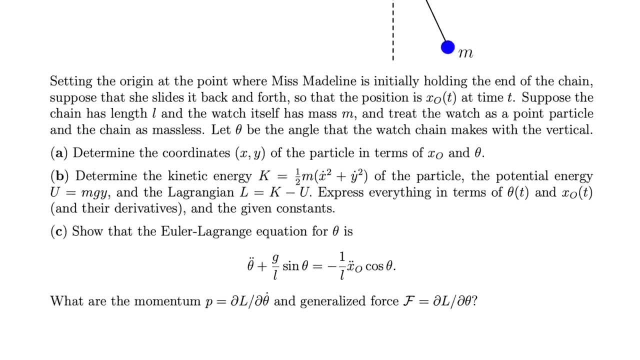 Now, if you really want to master these ideas, you've got to solve problems for yourself. So I've posted a problem sheet down below where you can apply the Lagrangian method to a challenging system. It's our pendulum again, this time in the guise of a pocket watch with magical powers. 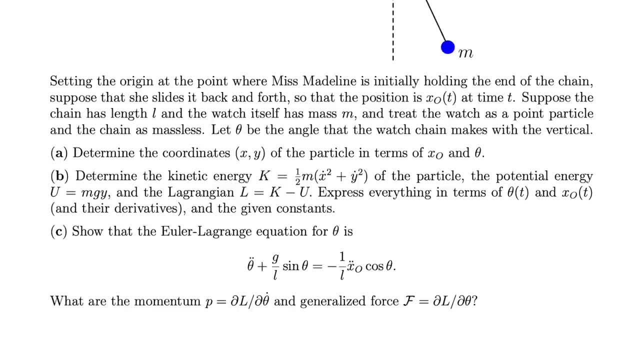 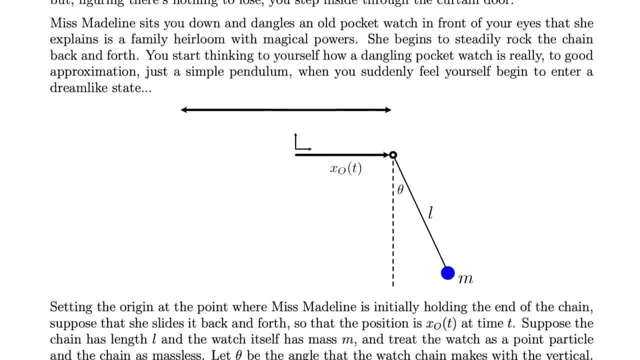 And now the pivot is being shaken back and forth by a mysterious hypnotist that you bump into at the town fair. So you should definitely go work that problem out to test and deepen your understanding, And I've also posted a link to the solutions which are available on my website. 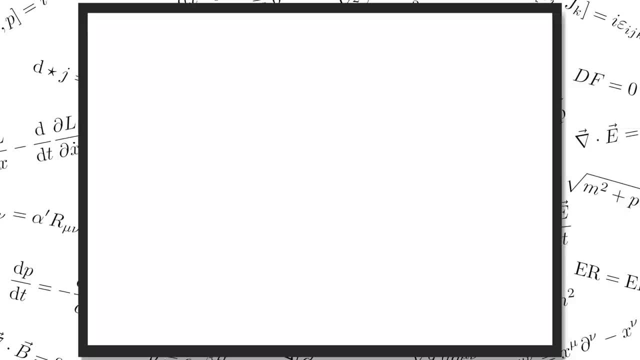 Finally, let's look at the pendulum using Hamiltonian mechanics. This time, instead of starting with the Lagrangian k minus u, let's write down the total energy k plus u For the pendulum. we get one half ml squared theta dot squared minus mgl cosine theta. 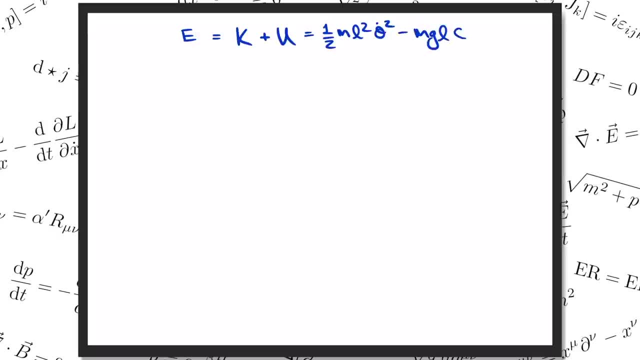 That minus sign is again there because the potential was negative. Now, remember that we defined the momentum p by ml squared theta dot. I'm going to use that expression to rewrite the first term in the energy as p squared over 2 ml squared, That means we can write the total energy in terms of theta and p. 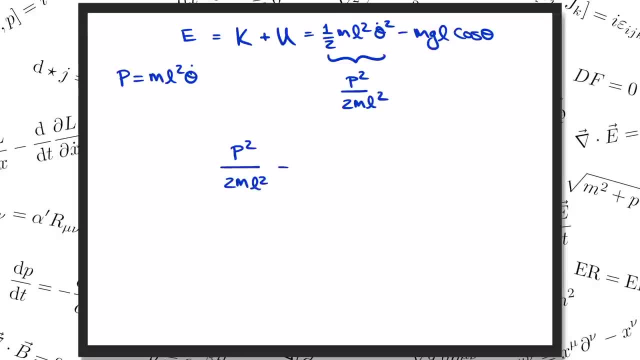 as p squared over 2 ml squared minus mgl cosine theta, This quantity is called the Hamiltonian and it's the starting point for Hamiltonian mechanics, just as the Lagrangian was the starting point for Lagrangian mechanics, Whereas we used the Lagrangian to write down the Euler-Lagrange equation. 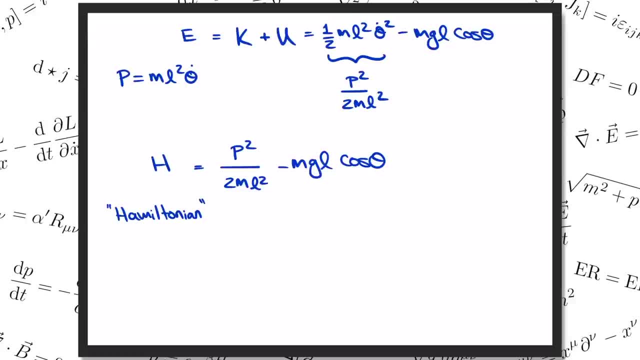 we'll use the Hamiltonian to write Hamilton's equations, which say that theta dot equals the derivative of h with respect to p, while p dot is equal to minus the derivative of h with respect to theta. Note that whereas F equals mA and the Euler-Lagrange equation, 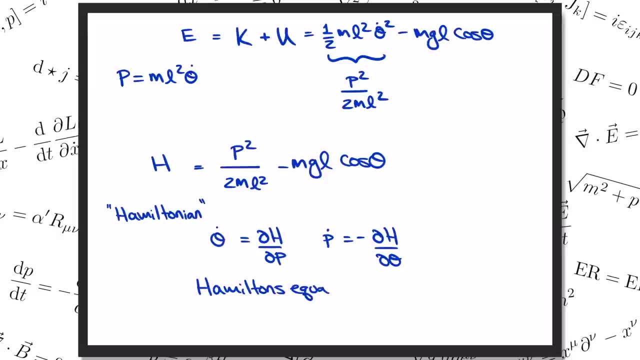 gave us a single second-order differential equation. Hamilton gives us a pair of equations which are called Lagrangian equations, Whereas we use the Lagrangian to write down the Euler-Lagrange equation. pair of first order equations for theta and p. 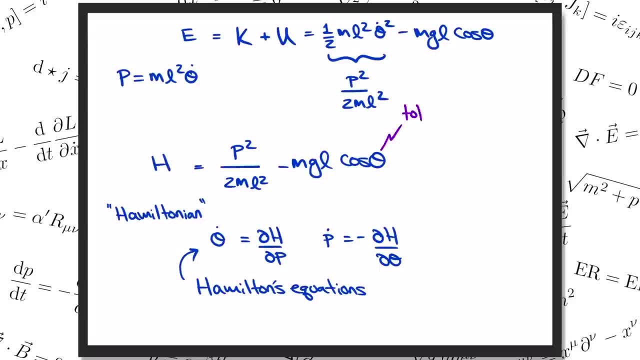 By the way, it's important to mention here that while the Hamiltonian was just the total energy in this simple example, that's not always necessarily the case. So let me give you the completely general definition before we move on. Remember that the momentum p was defined as the derivative of L with respect to the velocity. 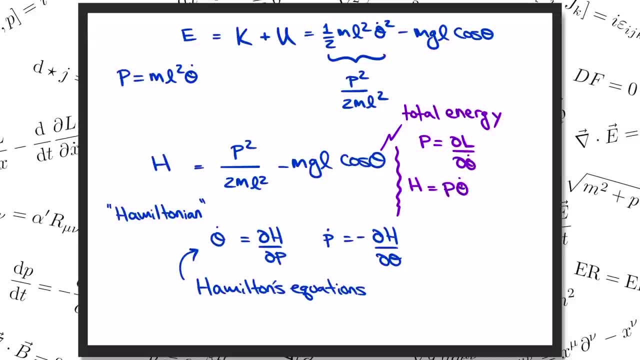 The Hamiltonian is defined by taking p times the velocity, and then subtracting L, And then, as before, you replace all the theta dots with p's. Now that may look like it comes out of left field and I don't have time to explain it. 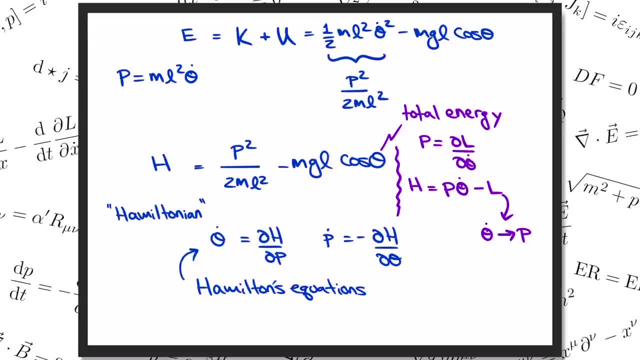 right now. but you can check that this definition reproduces the total energy in our pendulum example. But in the system I asked you to solve on the problem sheet, you're going to need this more general definition. So let's see what we get for our simple pendulum. 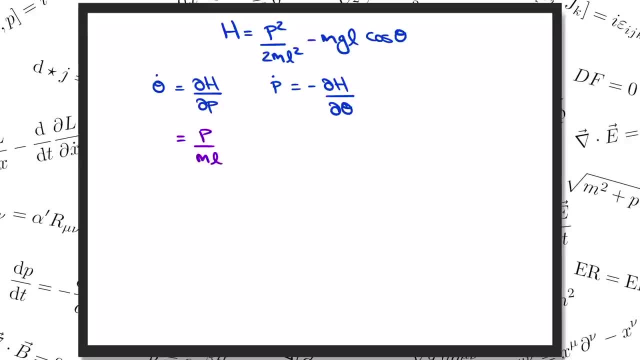 The derivative of h with respect to p is just p over mL squared from the first term. For the derivative with respect to theta, we get minus sine theta from the derivative of cosine times two. more minus sines gives us an overall minus mgl sine theta. 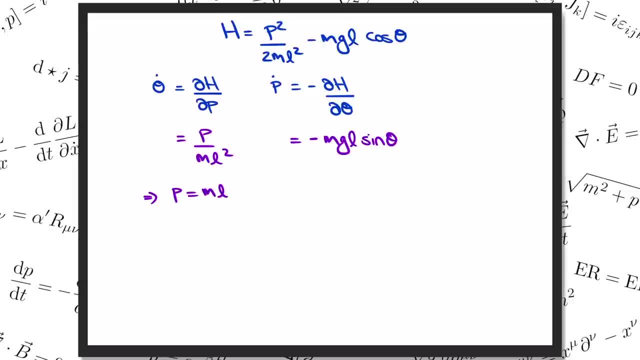 So Hamilton's equations tell us that p equals mL squared theta dot, and p dot is equal to minus mgl sine theta. This first equation is just the definition of momentum. again, If I take its rate of change, it says that p dot equals mL squared theta double dot. 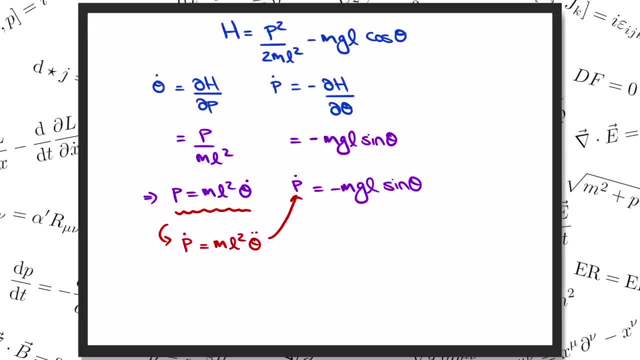 Now, if I insert that into Hamilton's second equation, we learn that mL squared theta double dot is equal to minus mgl sine theta. Crossing out the common factors, we arrive one more time at our old friend: theta double dot equals minus g over L sine theta. 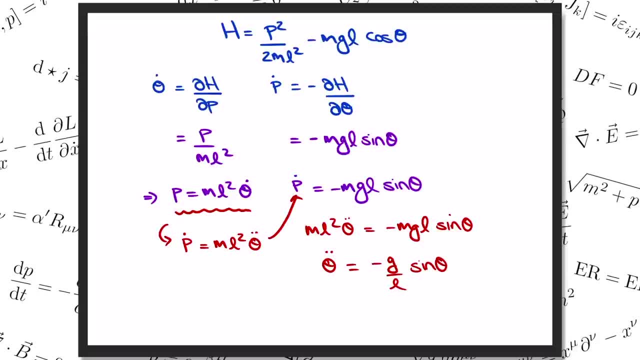 So if I take its rate of change, it says that p dot equals mL squared theta double dot. So Hamilton's equations are equivalent to the original equation of motion that we got either from f equals mA or from the Euler-Lagrange equation. 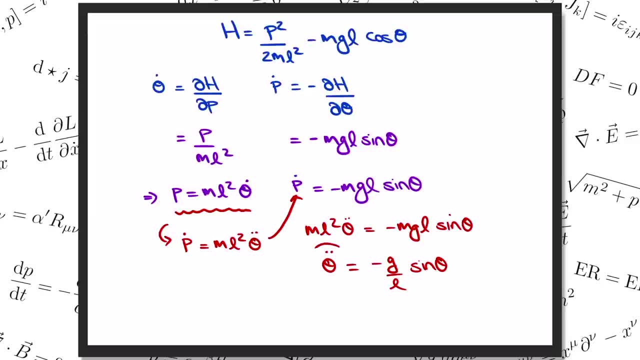 They just split the single second order differential equation into a pair of first order equations. first order because we only have one derivative acting on theta and p. But what does that really buy us? Hamilton's pair of first order equations aren't necessarily any easier to solve than 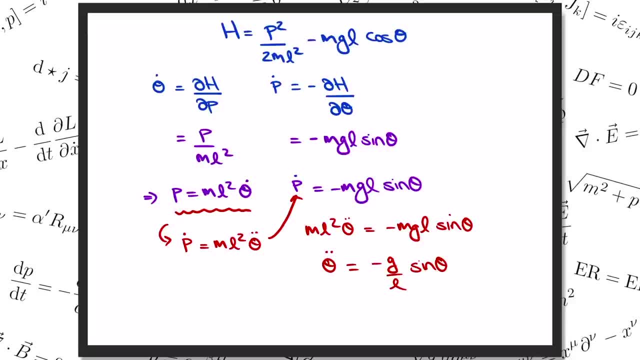 the single second order equation of motion that we started with. Now, what we do gain is that we can do that even if we don't have the same number of equations. however, is a new geometric perspective on the mechanics of the pendulum by connecting 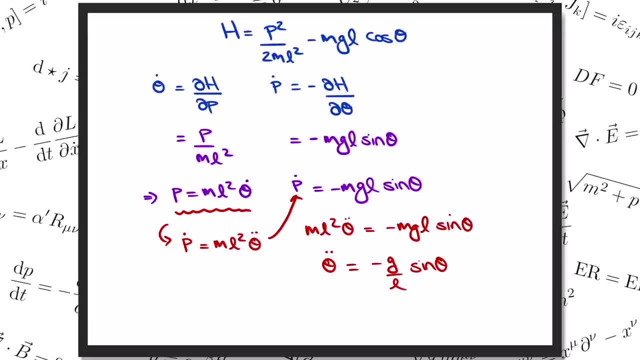 it to what's known as a flow on phase space, as I'll now explain. To specify what the pendulum is doing at any given instant in time, we just need to give its position and velocity or, equivalently, its position and momentum, theta and p. 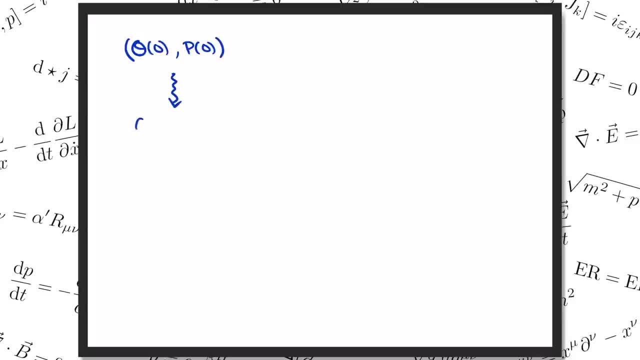 With this initial data we can figure out what the pendulum will be doing at any later time. by solving Hamilton's equations for theta of t and p of t, The pairs of thetas and p's define a plane which is called the phase space of the system. 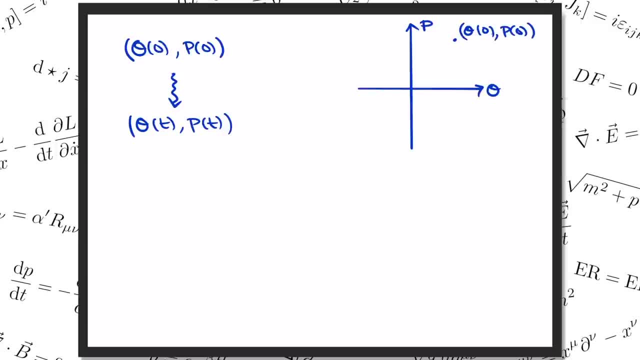 We start out at our initial condition: theta of zero, p of zero. and as time goes on, our coordinate moves around this theta, p plane tracing out a curve which is known as a flow on this phase space. These flows are very special. they won't just travel along any old curve in the theta. 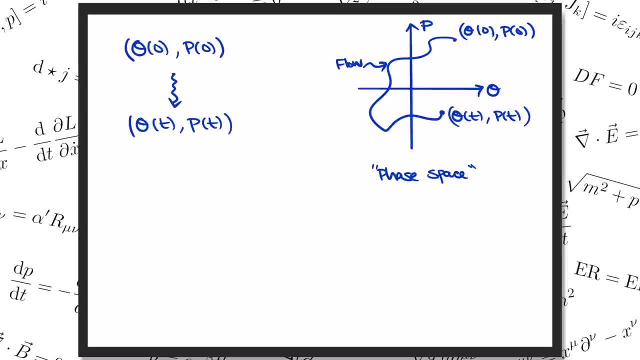 p plane, In particular because the energy of the pendulum is constant. the energy of the pendulum is served. If we evaluate the Hamiltonian at any time, t along the flow, we're guaranteed to always get the same number. The energy is a constant of the flow. 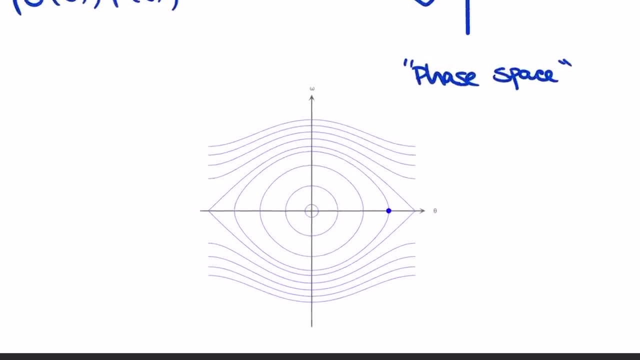 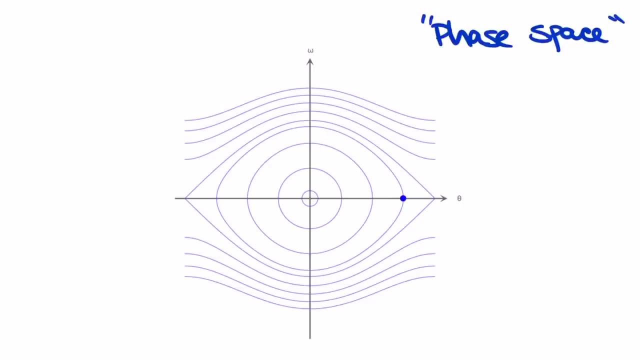 Here's what a few of the lines of constant energy look like for our pendulum. Because the energy of the pendulum is constant, we know that our initial point has got to move along one of these lines of constant energy as it evolves with time. 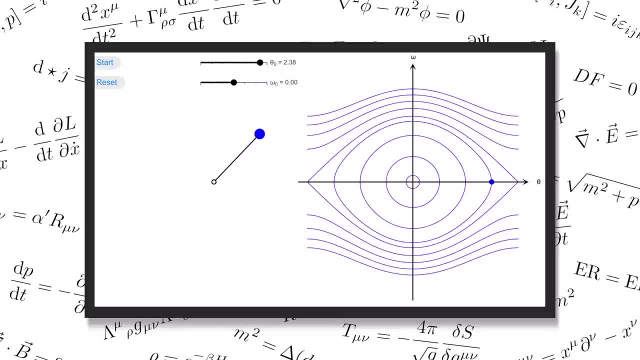 So here's another little animation that I made. Again, you drag these sliders to set the initial conditions that you want. You can see that the energy of the pendulum is constant. So here's another little animation that I made. You can see that the energy of the pendulum is constant. 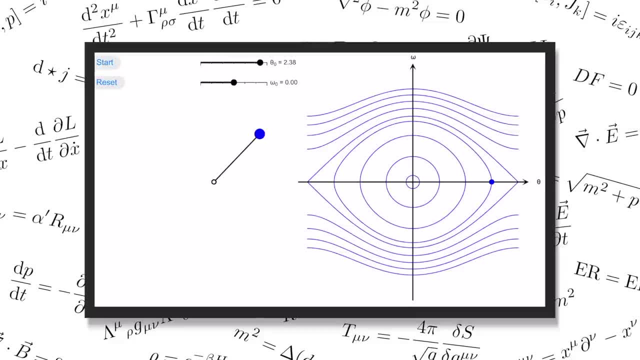 The initial conditions. pick out your starting point in the phase space. So I'm starting out with some particular angle and zero momentum. Then we're going to let the pendulum go and see how it evolves with time. As the pendulum moves, its angle and angular velocity are changing with time and therefore 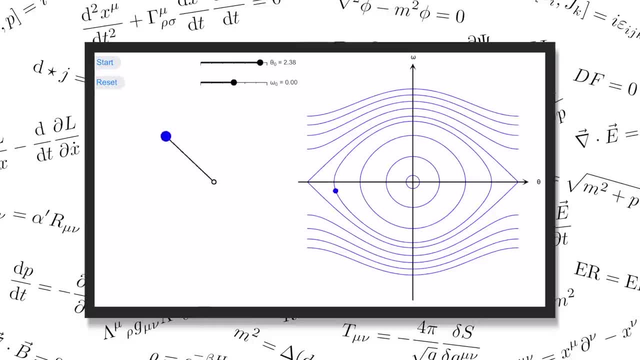 the phase space coordinate is changing, But since the energy is constant, we know that the particle has got to travel along along this line of constant energy. So, again, I'll put a link to this little animation down below so that you can go play with it. 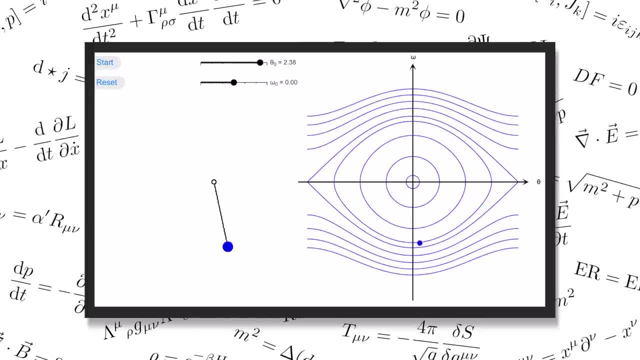 for yourself. Notice in particular that there are these two different kinds of curves of constant energy. We've got these closed loops near the center of the phase space and these open wavy lines farther away. Try setting the initial conditions so that the particle sits on one of the wavy lines. 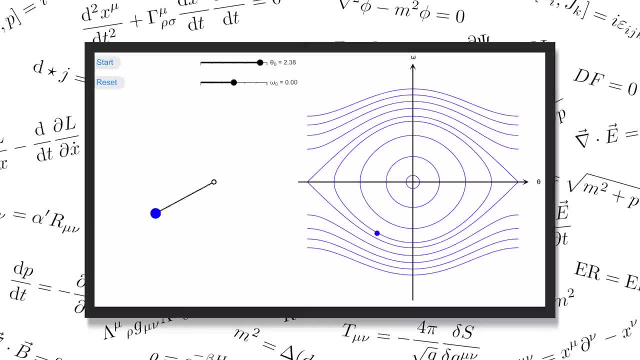 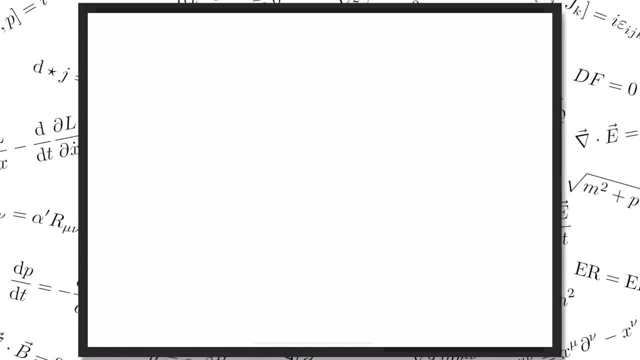 and figure out what the physical difference is between these two types of phase space flows. All this is only the tip of the iceberg for Lagrangian and Hamiltonian mechanics and I'm really hoping that I've whet your appetite to make you curious to go off and learn more.